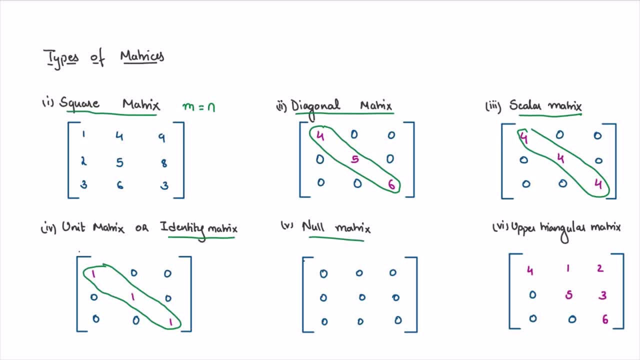 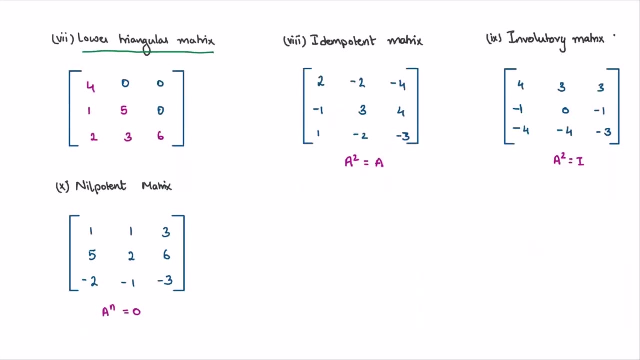 The fifth type of matrix is null matrix. In this, all the elements are equal to 0. The sixth type of matrix is upper triangular matrix. In this, all the elements below the diagonal are equal to 0.. The seventh type of matrix is lower triangular matrix. 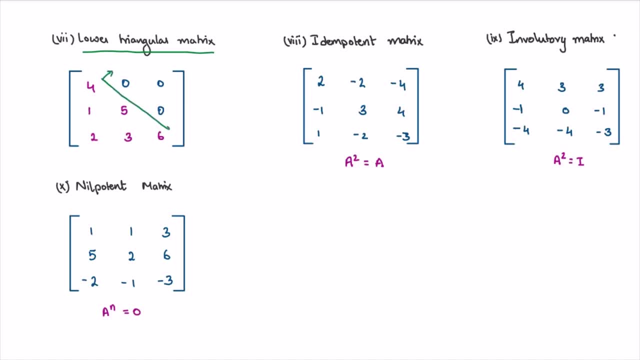 where all the elements above the diagonal are equal to 0.. The eighth type of matrix is idempotent matrix where square of matrix A is equal to A. The ninth type of matrix is involuntary matrix where A square is equal to I. 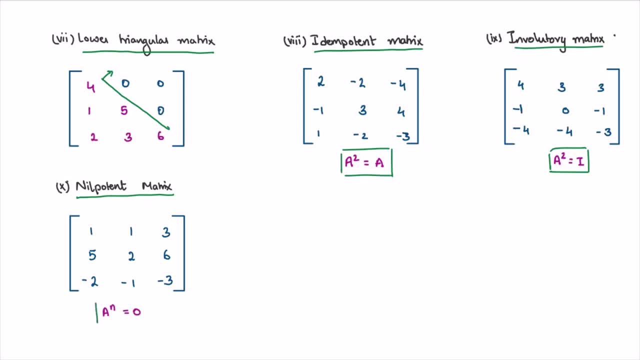 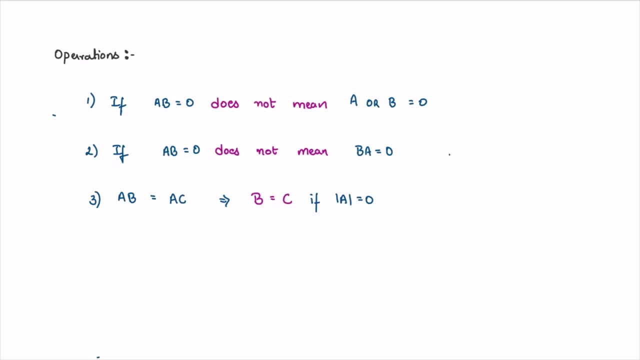 The last type of matrix is nilpotent matrix, where A to the power of n is equal to 0.. Now there are some operations which you need to remember. If matrix A multiplied by B is equal to 0,, then it doesn't mean that 1 of A or B is equal to 0.. 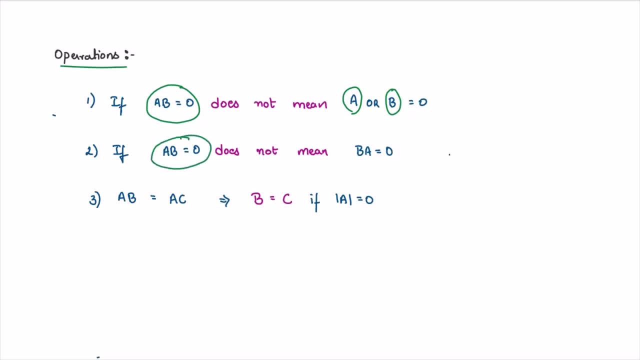 Also, if AB is equal to 0,, then it does not mean that BA is equal to 0.. The third operation is: if AB is equal to AC, then B is equal to C if determinant of A is not equal to 0.. 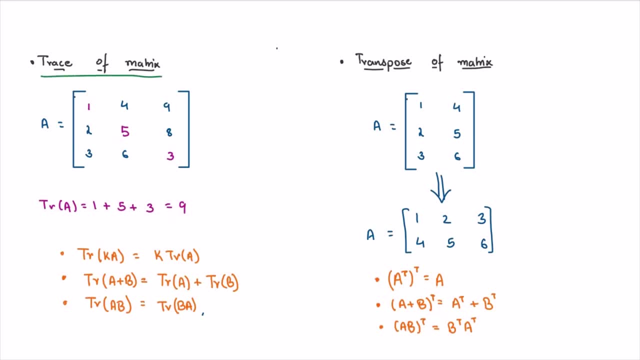 Now let us come to trace of matrix. The trace of matrix is given by sum of diagonal elements. For this matrix, diagonal elements are 1 plus 5 plus 3, which is equal to 9.. We have some properties of trace of matrix. 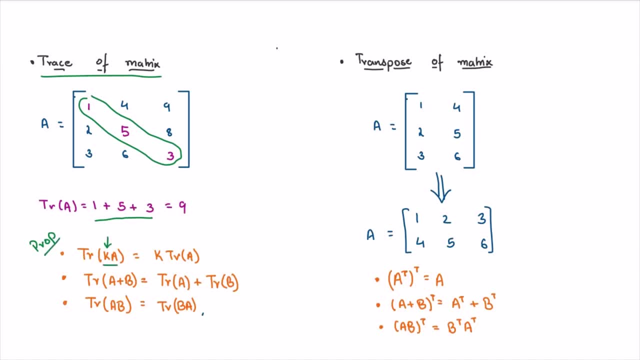 If K is a scalar trace of matrix KA is equal to K multiplied by trace of matrix. The second property is: trace of matrix A plus B is equal to trace of matrix A plus trace of matrix B. The third property is: trace of matrix A multiplied by B is equal to. 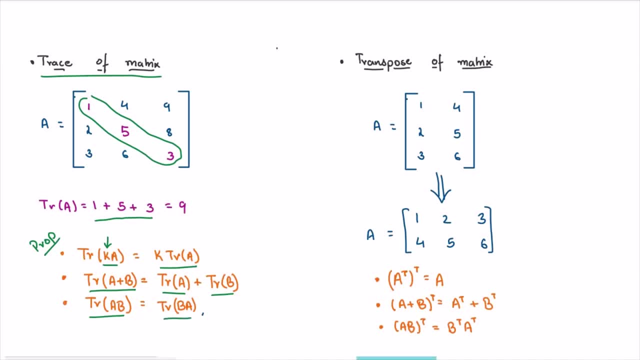 trace of matrix B multiplied by A. Next term is transpose of matrix. Transpose of matrix means converting rows into columns, as we have done for this matrix. Now, properties of transpose of matrix are: transpose of A. transpose is equal to A. The second property is: 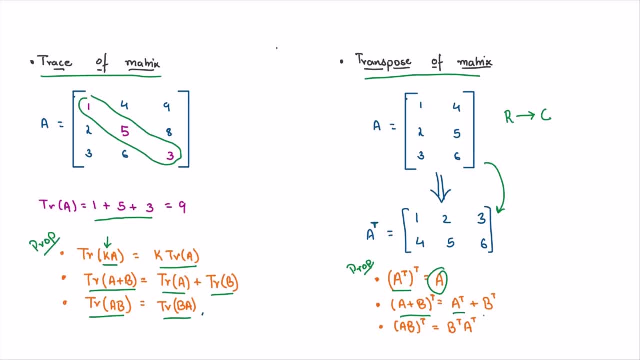 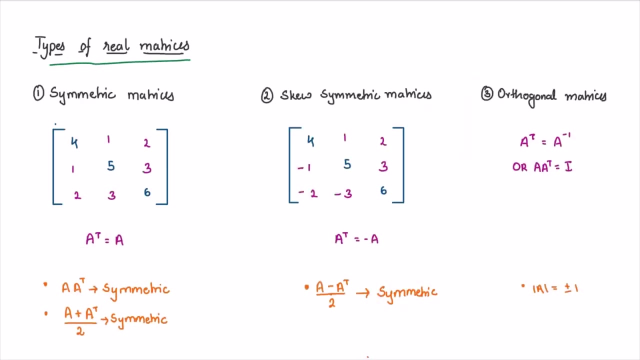 A plus B whole transpose is equal to A transpose plus B transpose. And the third property is A multiplied by B whole transpose is equal to B transpose multiplied by A transpose. Now coming to types of real matrices, There are three types of real matrices. 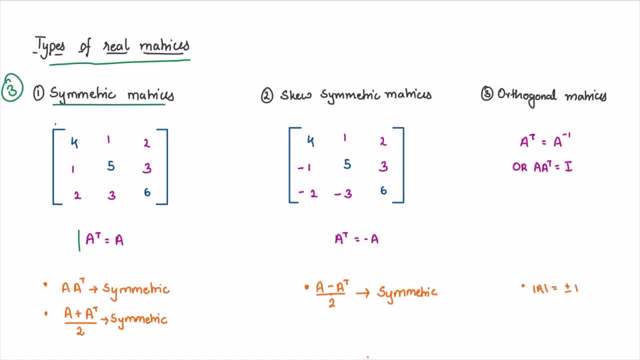 The first one is symmetric matrices where A transpose is equal to A. You see, elements above the diagonal are equal to elements below the diagonal And there are some properties Matrix: A multiplied by A transpose is always symmetric. Also, A plus A transpose by 2 is always symmetric. 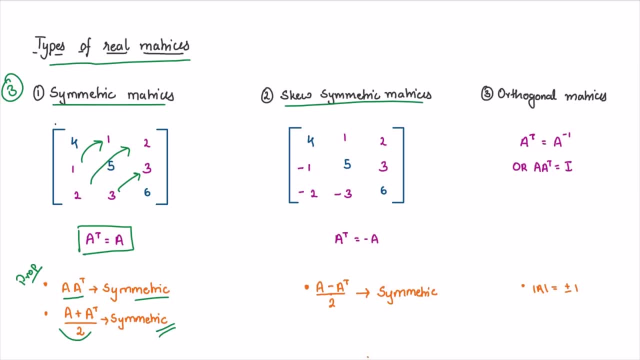 The second type of real matrices are skew symmetric matrix. In this A transpose is equal to minus A. Observe that in this matrix the elements above the diagonal are negative of element below the diagonal And the property of skew symmetric matrices is A minus A transpose by 2. 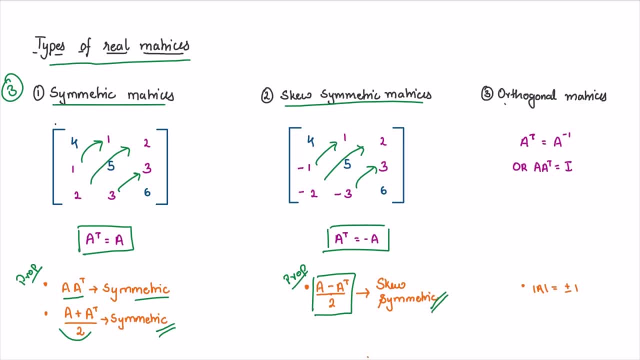 is always skew symmetric. The third type of real matrices is orthogonal matrices, where transpose of matrix A is equal to inverse of matrix And the determinant of orthogonal matrix is always plus or minus 1.. Now let us learn two more operations. The conjugate of matrix is: 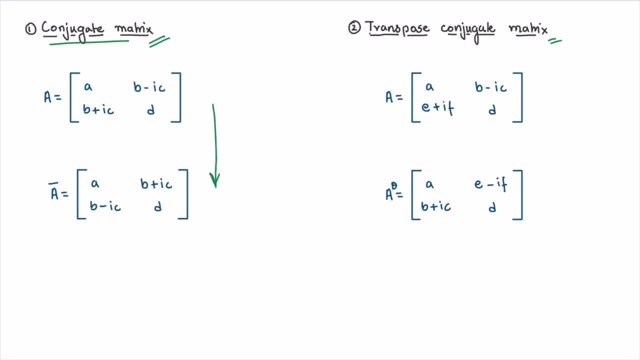 conjugate of each element of a matrix where we change the sign of imaginary terms And the transpose conjugate matrix is transpose of conjugate matrix. The conjugate of matrix Ae is this and the transpose of this matrix is transpose conjugate matrix. Now coming to types of complex matrices, 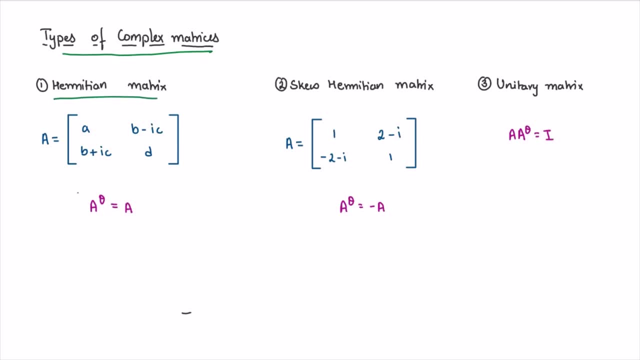 The first type of matrix is Hermitian matrix, where transpose conjugate of matrix A is equal to A. The next type of matrix is skew Hermitian matrix, where transpose conjugate of matrix A is equal to minus A. And the last type of matrix is: 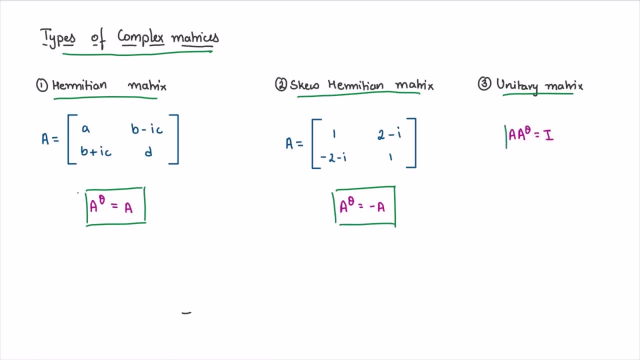 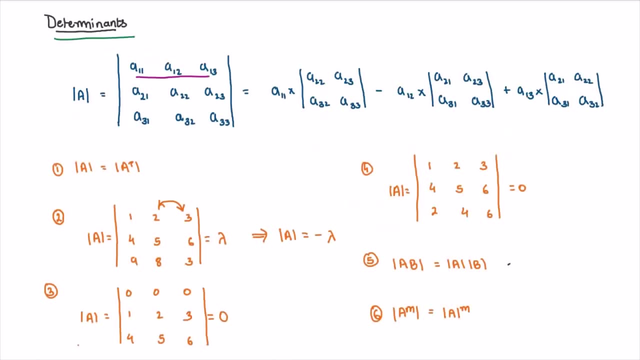 unitary matrix where A multiplied by transpose conjugate of matrix A is equal to. I Now coming to determinant of matrix. For a 3x3 matrix, determinant above this line can be given in this way And move on to properties of determinants. 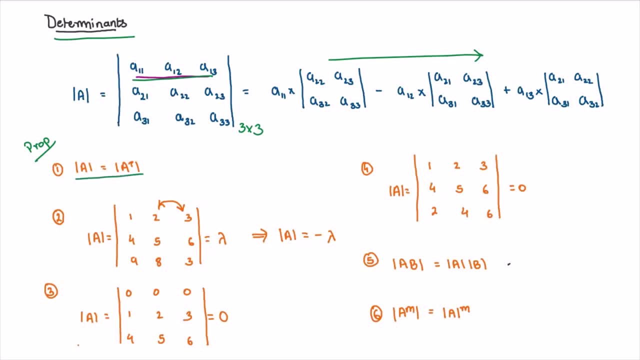 The first property is: determinant of matrix A is equal to determinant of matrix A transpose. The second property is: if we interchange two rows or columns of a matrix, determinant is multiplied by minus 1.. The third property is: if any one row or column of a matrix is equal to 0. 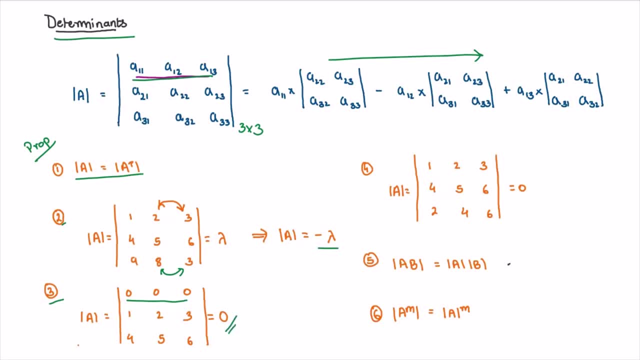 then determinant of a matrix is equal to 0.. The fourth property is: if any two rows or column of a matrix are proportional, then determinant of a matrix is equal to 0.. The fifth property is determinant of a matrix: A multiplied by B is equal to. 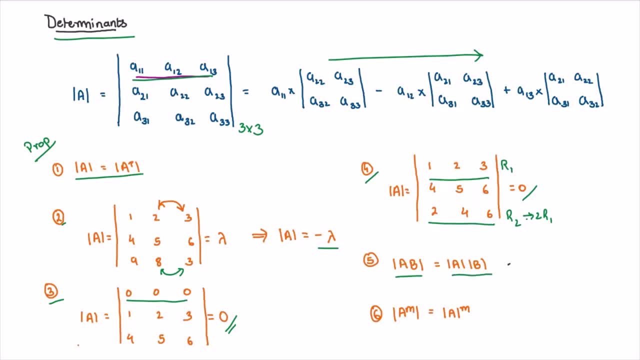 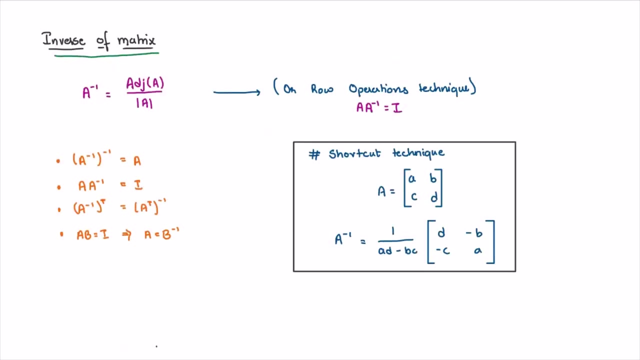 determinant of A multiplied by determinant of B. The sixth property is: determinant of A to the power of M is equal to determinant of matrix A to the power of M. Next topic is inverse of matrix. Inverse of matrix exists only when determinant of A is not equal to 0.. 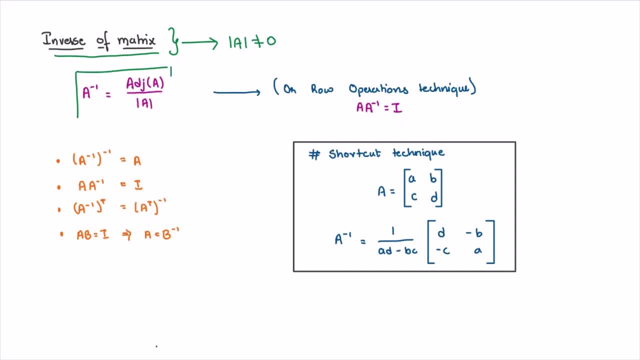 To find the inverse of matrix we can use the formula A, inverse equal to adjoint of A by determinant of A. We also have an alternate to find the inverse using row operations technique. For that we use the formula A into A inverse equal to I. 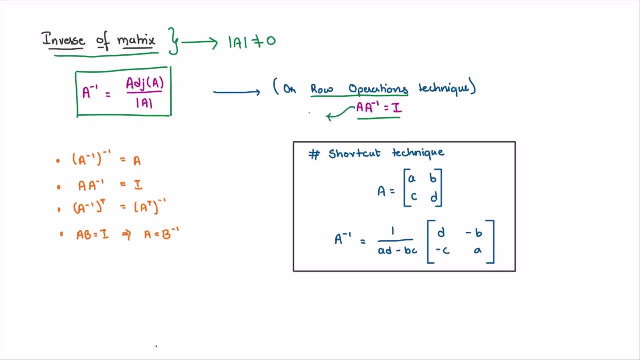 Where we convert this A into identity matrix using row operations and the resulting right hand side will give us A inverse. For a 2x2 matrix, we have a shortcut formula, A inverse equal to 1 by multiplied by matrix, and the properties of inverse of matrix are: 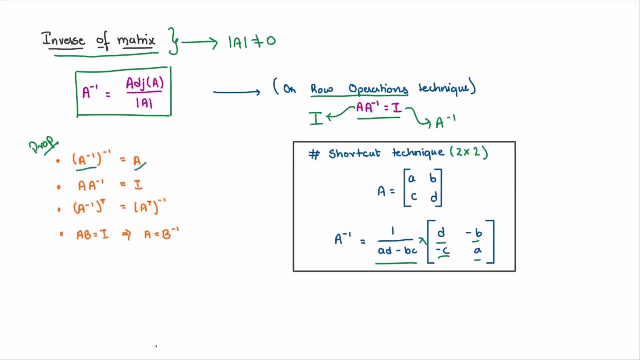 the inverse of A inverse is equal to A. A multiplied by A inverse is equal to I. The transpose of A inverse is equal to inverse of A transpose. and the last property is: if A multiplied by B is equal to I, then A is equal to B inverse. 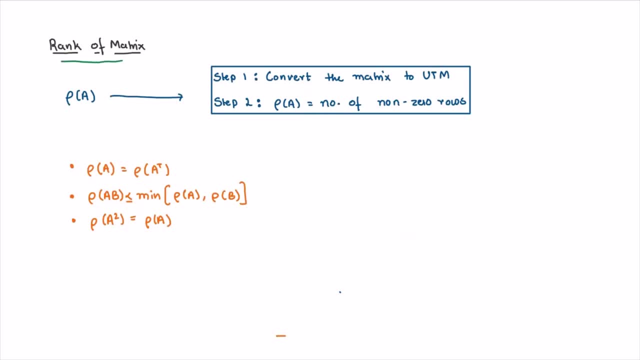 The next topic is rank of matrix. To find the rank of matrix, first convert the matrix into upper triangular matrix using row operations, and number of non-zero rows present in the resultant matrix is equal to rank of matrix. The properties of rank of matrix are: rank of matrix A. 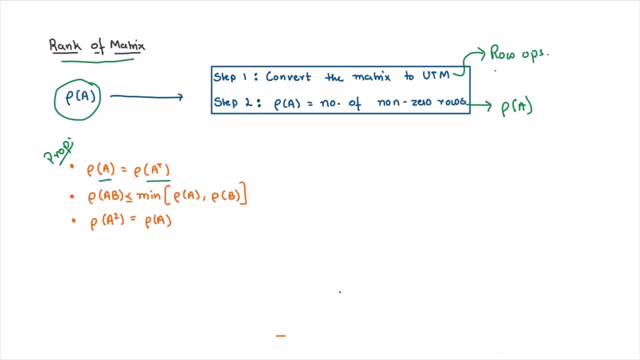 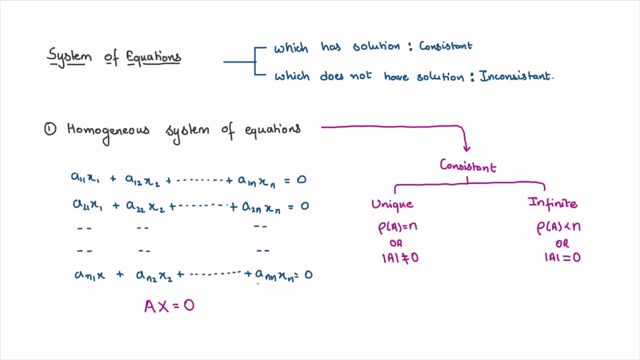 is equal to rank of A. transpose The rank of matrix: A multiplied by B is always less than or equal to minimum of rank of A or B. The last property is: rank of A square is equal to rank of A. The rank of A square is equal to rank of A or B. 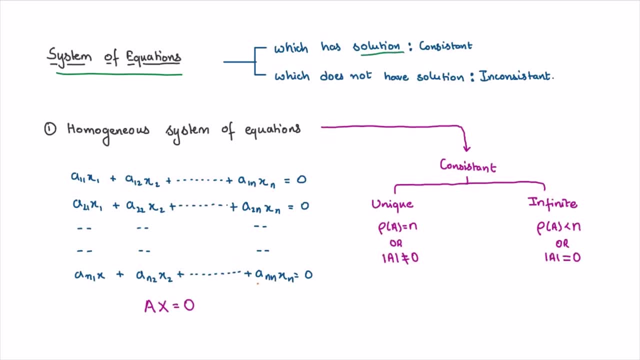 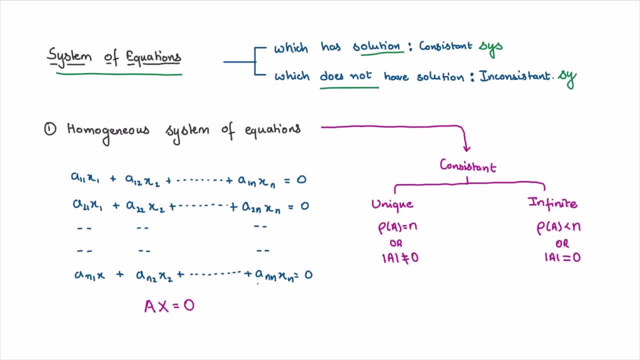 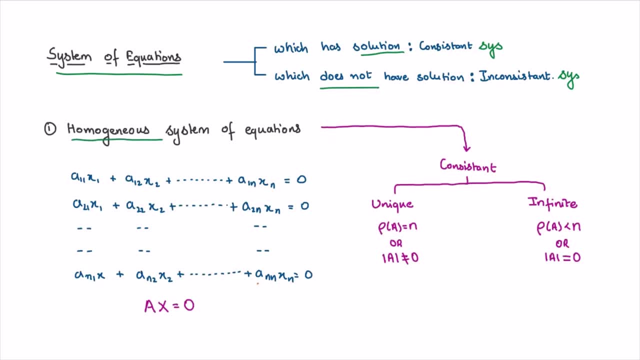 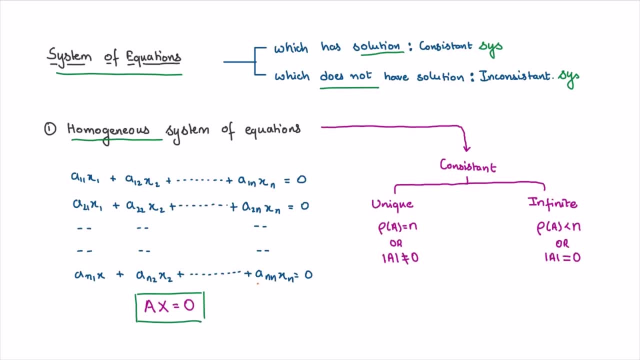 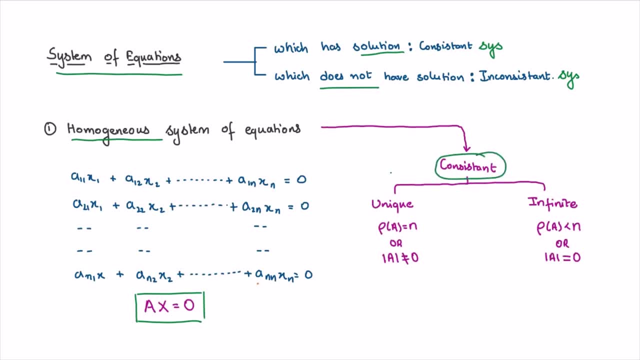 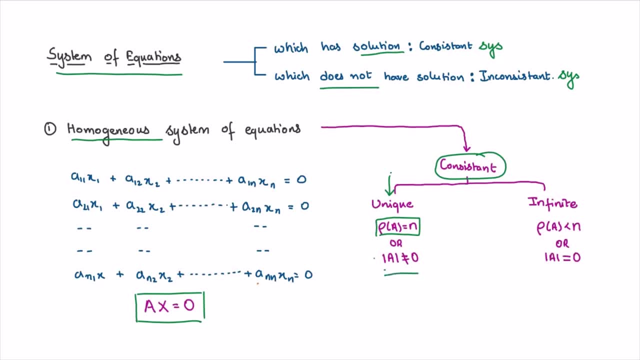 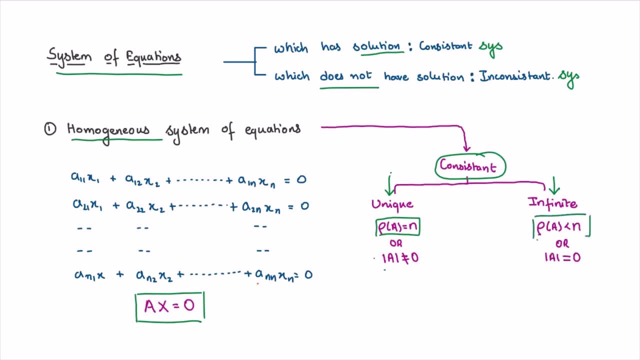 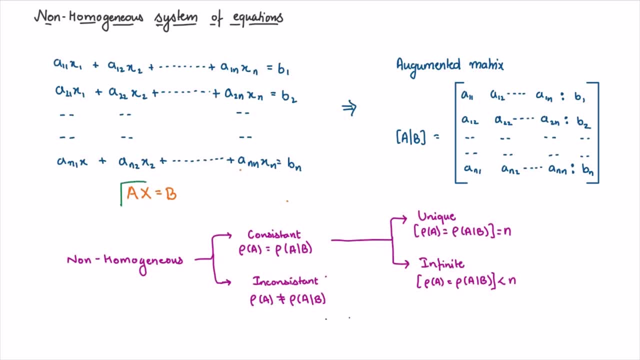 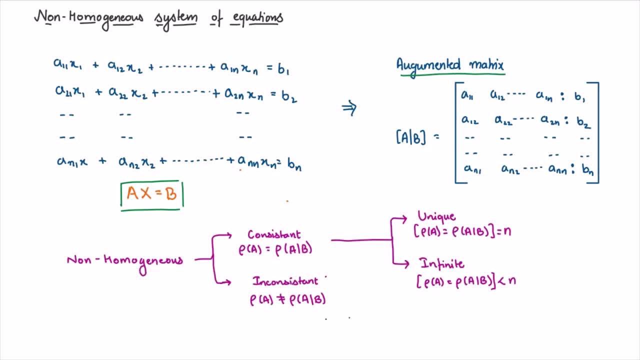 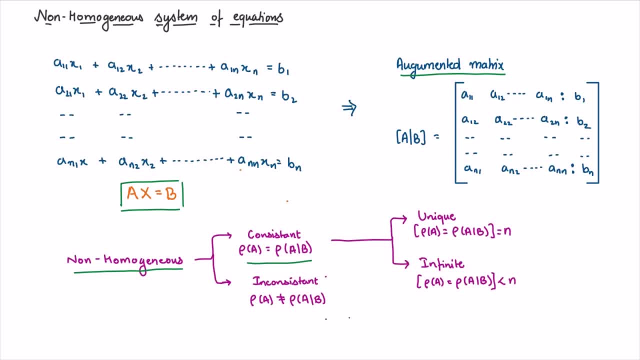 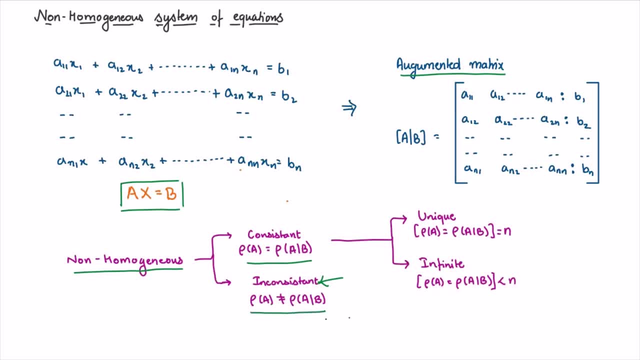 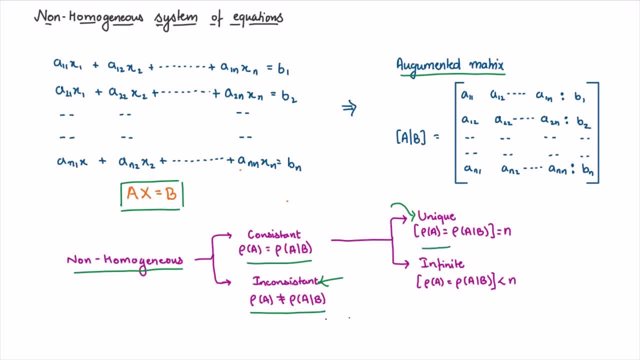 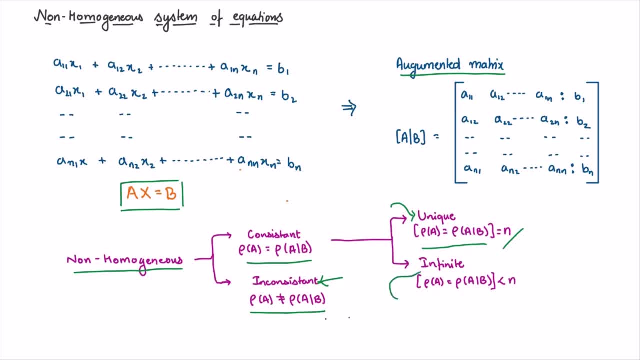 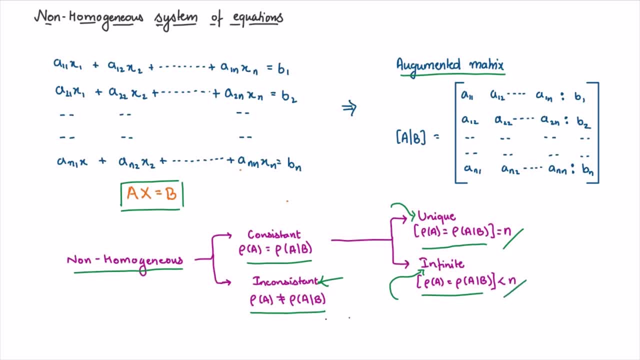 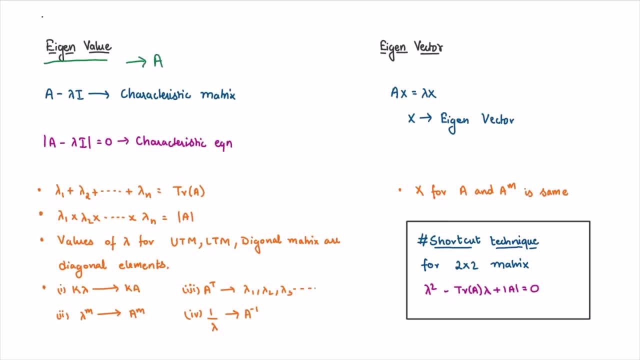 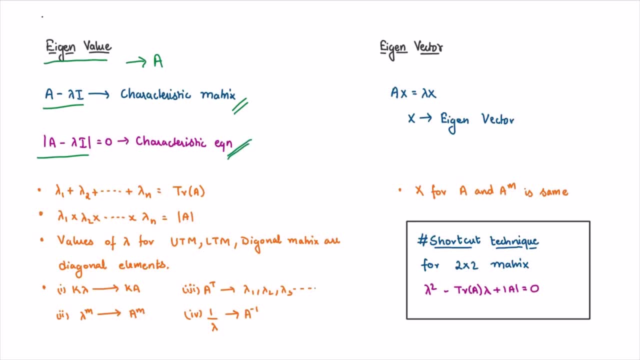 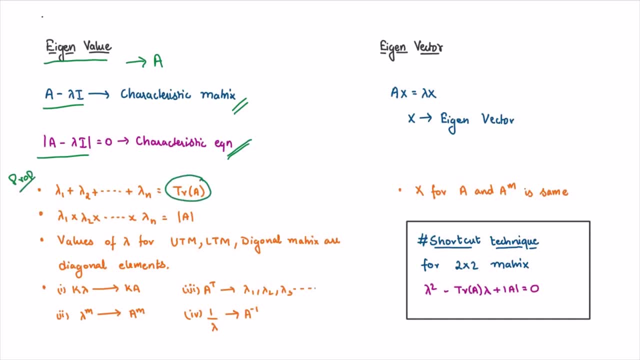 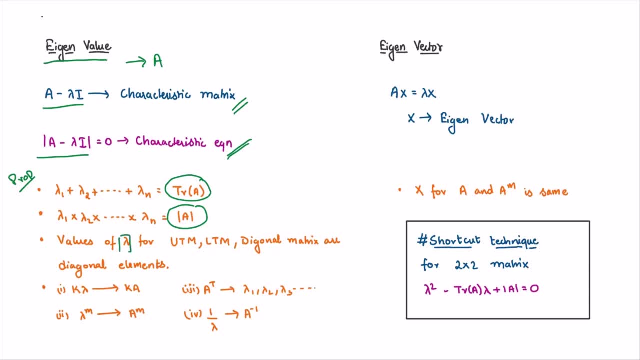 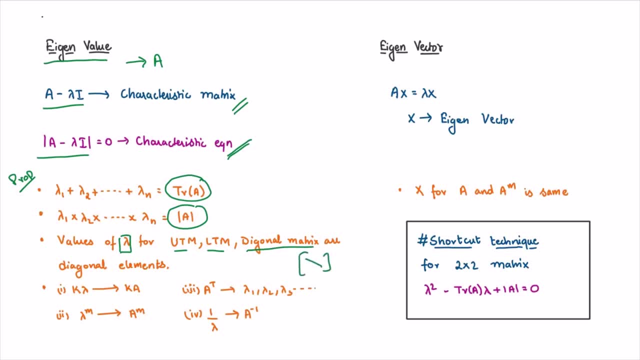 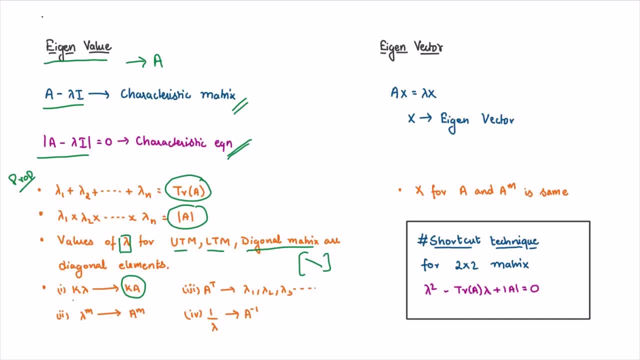 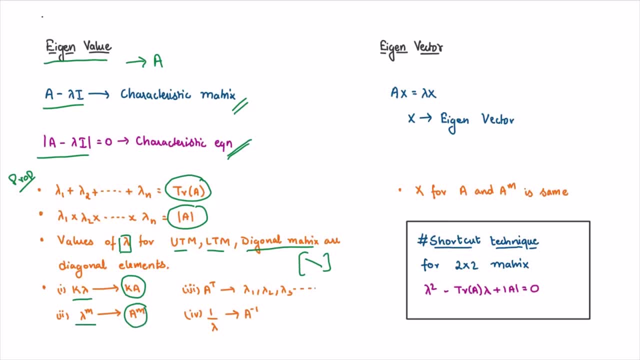 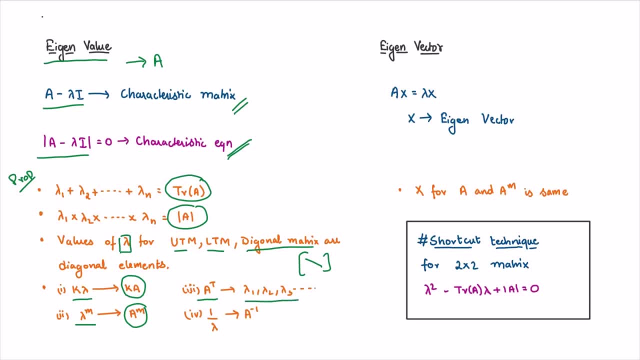 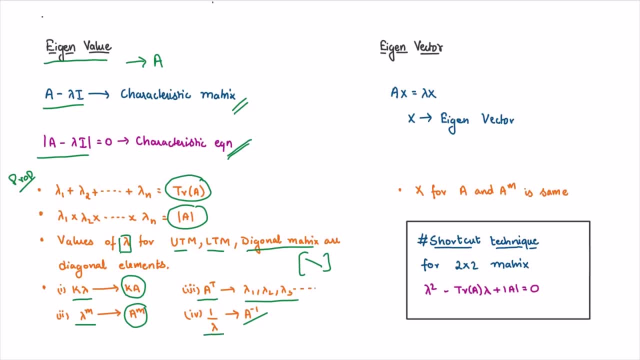 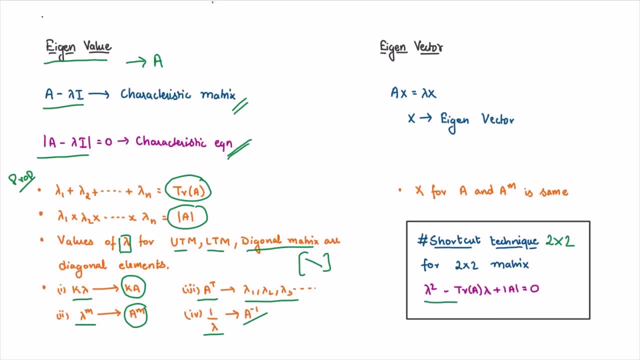 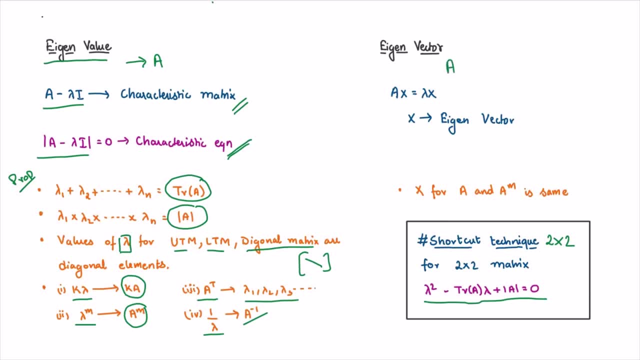 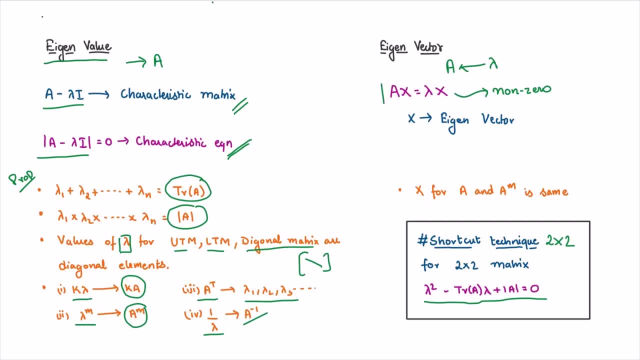 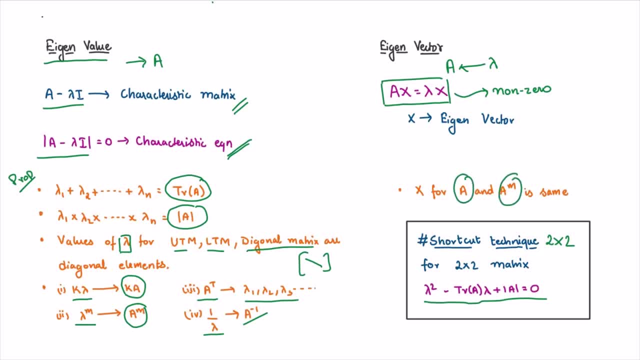 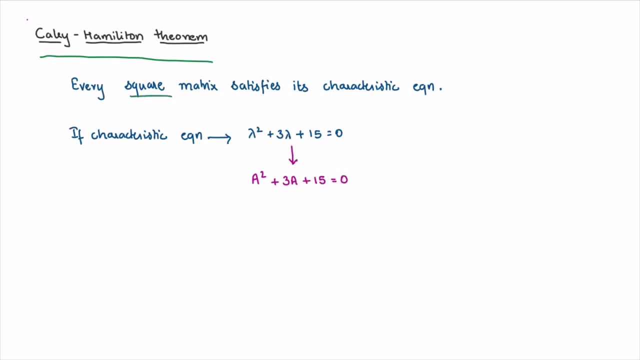